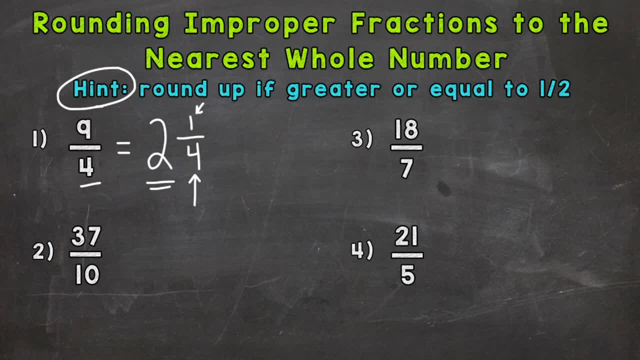 than a half. therefore, we stay the same as far as this whole number goes. So two and a fourth rounds to two. Now, this symbol here stands for close to or approximately, and we can use it when rounding. It's helpful when rounding because we don't want to use an equal sign, because two and 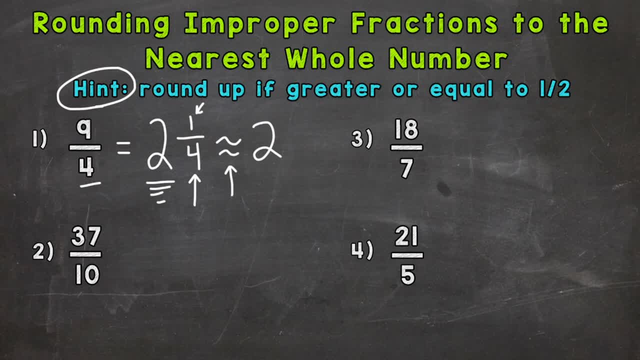 one fourth is not equal to two. It's close to or rounds to two. So let's move to number two, where we have 37 tenths. So first thing, we do convert to a mixed number. So we divide 37 divided by 10.. How many whole groups of 10 out of 37?? Well, three. That gets us to 30. So we have. 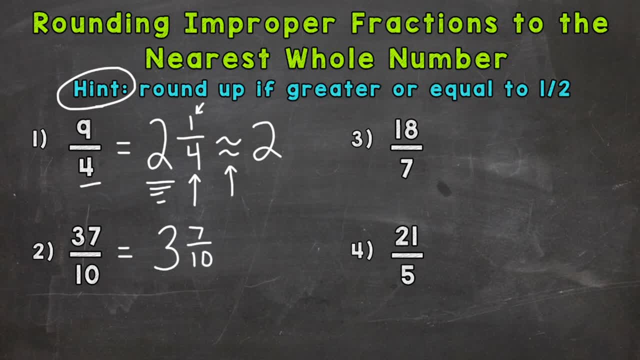 seven left over, and we keep our denominator of 10 the same. So now we're ready to round. So is three and seven tenths closer to two? No, it's closer to two. So we divide 37 divided by 10.. So 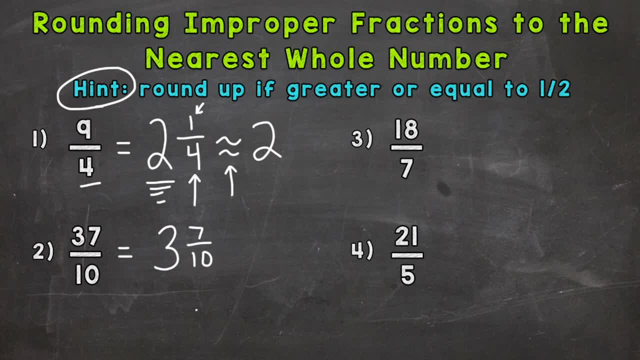 is three and seven tenths closer to three, Or is it closer to four? Let's take a look at our fractional part here. Seven tenths- Well, we know five tenths is half, so seven tenths is greater than half. Therefore, we round up: Three and seven tenths rounds to four. It's closer to four. 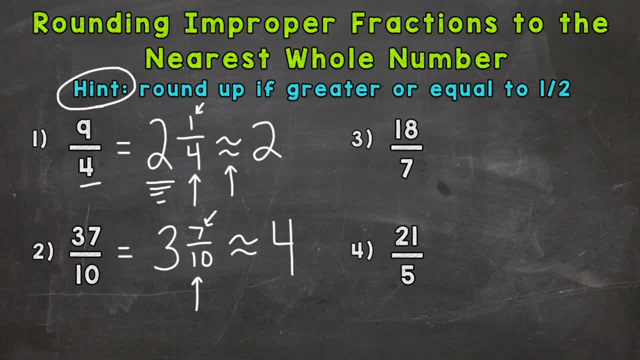 than it is to three. On to number three: we have 18 sevenths. So let's convert to a mixed number here. How many whole groups of seven out of 18?? Well, two, That gets us to 14.. So we have four. 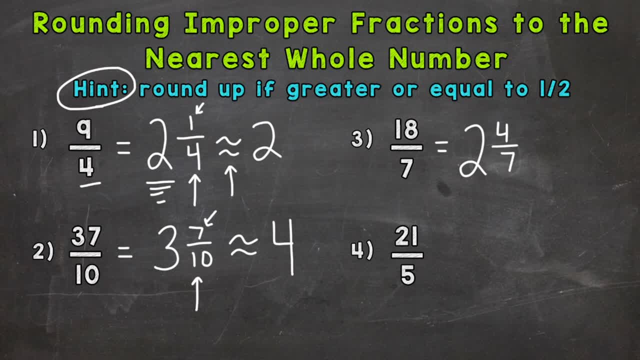 left over. Keep the denominator of seven the same. So two and four sevenths. So let's see Three and a half is half of seven. So this four is a little more than half. So we do round up. So two and four sevenths rounds to three. And lastly number four, we have 21 fifths. 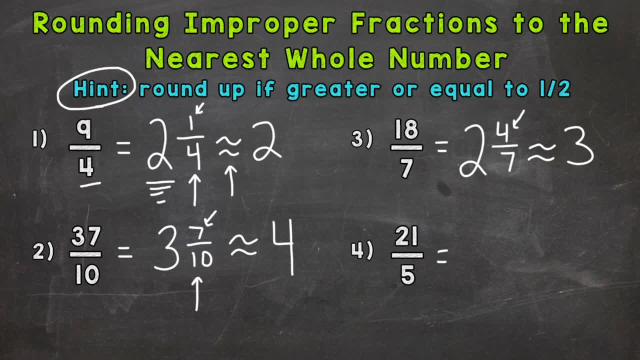 So let's convert to a mixed number. How many whole groups of five out of 21?? Well, four, And we have one left over, because five groups of- I'm sorry, four groups of five gets us to 20.. We have a.